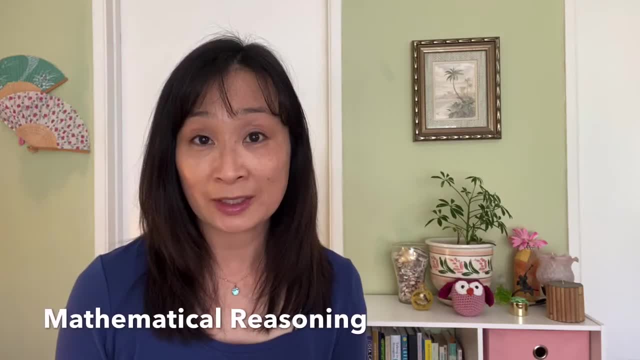 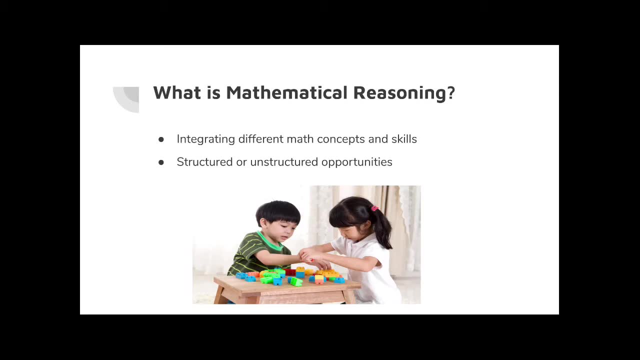 Mathematical reasoning is the fifth strand of math. So what is a mathematical reasoning? It's where you are now integrating all the different math concepts and skills together, and then it could be either through structured or unstructured opportunities. So, for example, if you wanted a child to count out the triangles, how many triangles do you see? So 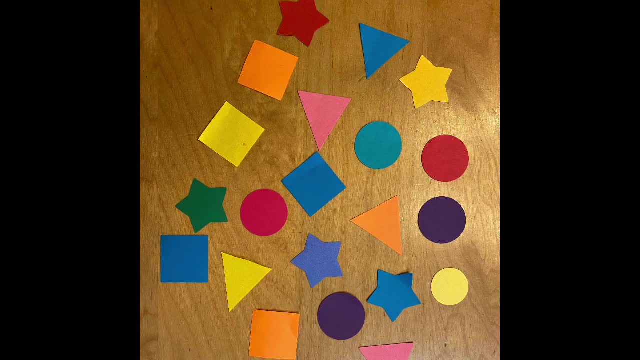 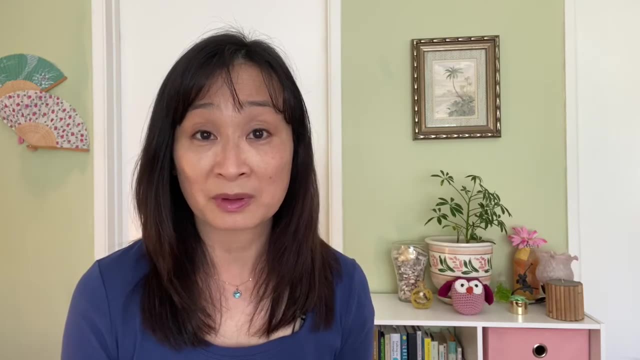 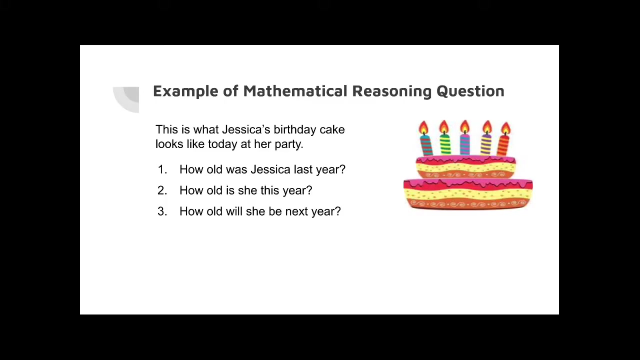 now they are applying number sense, counting and geometry by identifying the triangles. Mathematical reasoning is a great way for children to develop critical thinking skills and also to apply math to everyday situations. Here's an example of a mathematical reasoning question that you can ask a child. Show them a picture of a birthday cake and then say: 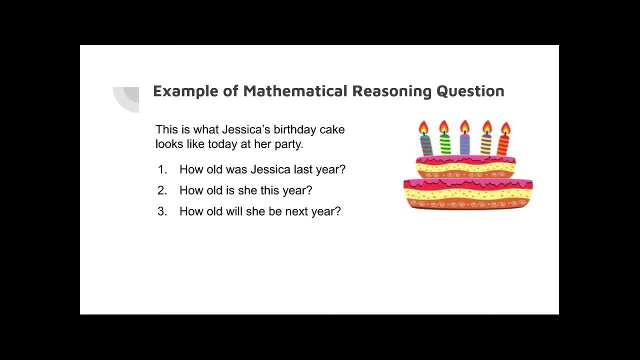 this is Jessica's birthday cake. This is what it looks like today at her party. So how old was Jessica last year? So which concept or which skill will the child need to be able to answer that? Well, first they have to be able to count, and then they have to know. last year means that they were younger. 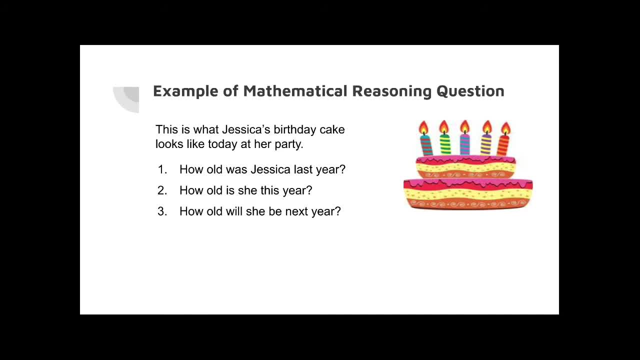 So they can count out. okay, there are five candles, So that means if there are five this year, they must be one less than five, four. And then you can ask how old is she this year? By the same, by counting and then associating the. 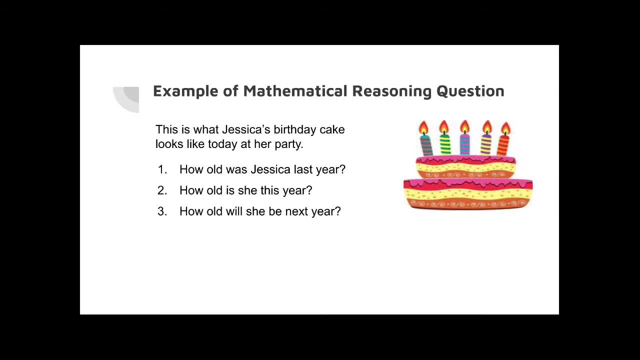 number of candles to her age this year, and then how old will she be next year? and so the concept that they will need to apply here is addition: like they'll another year, so next year from now there'll be another year older than they are today, so that would mean that they would be six years old, because it's one. 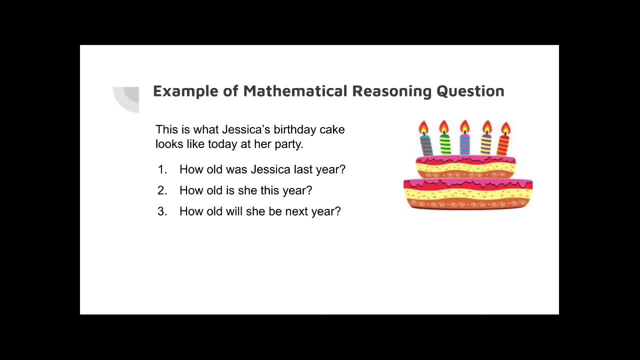 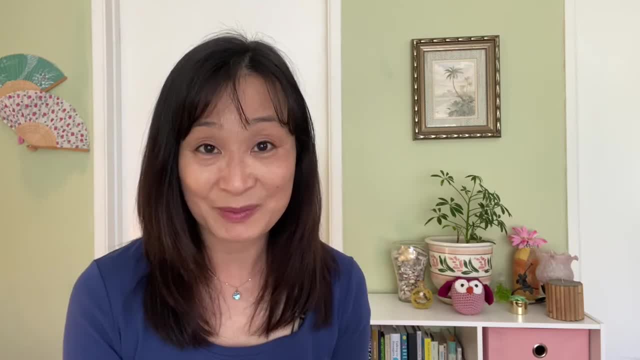 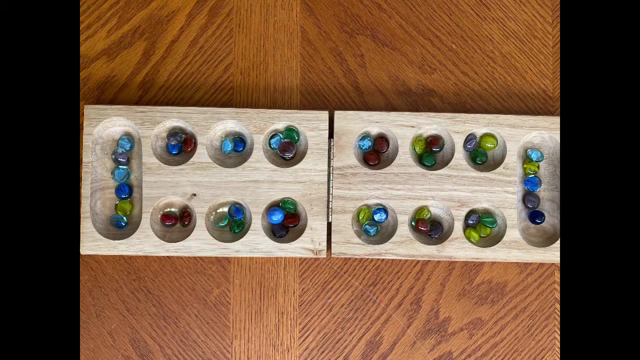 additional year from the number of candles that they see in this picture. a great way to help children develop mathematical reasoning in a fun way is playing games, so there's a lot of board games out there that kids love. I grew up with Candyland or chutes and ladder man Mancala. that's a classic where they need. 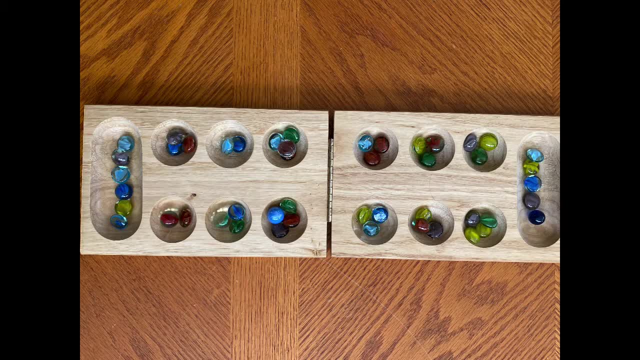 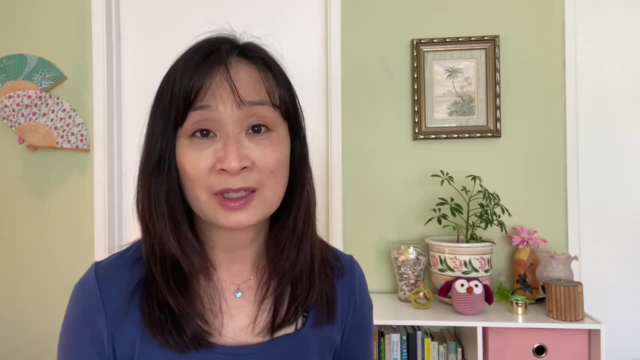 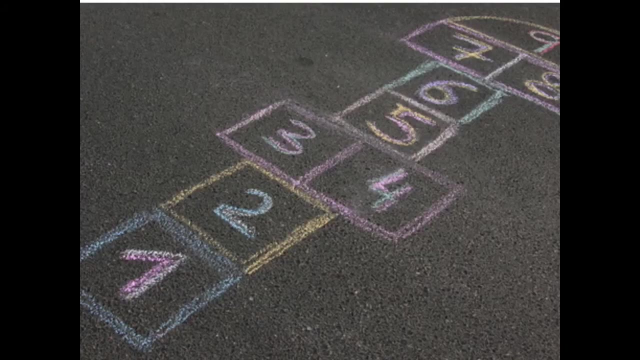 to count out the different marbles and Mancala. Candyland- their shapes involved, and then chutes and ladders- goes up and down, and so there's spatial relationships that are involved in that game. there's different card games that are really fun and there's a lot of games that you can play outside. so hopscotch, that's a.